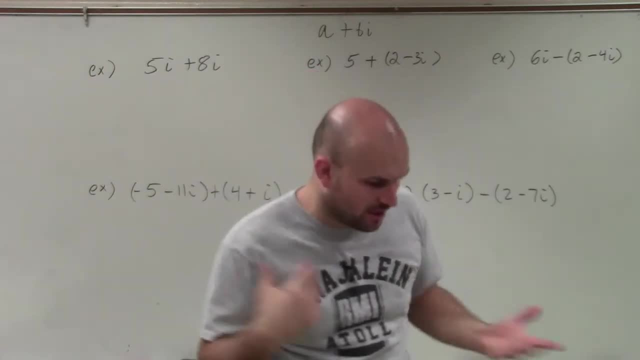 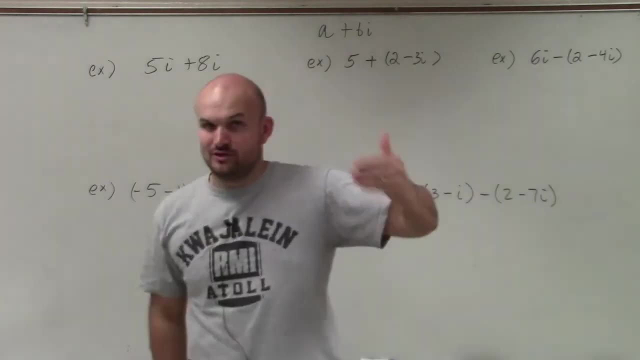 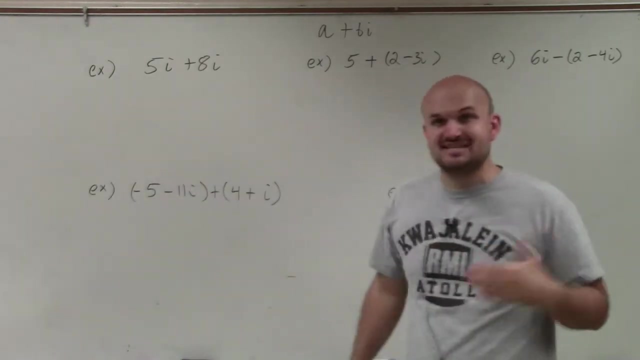 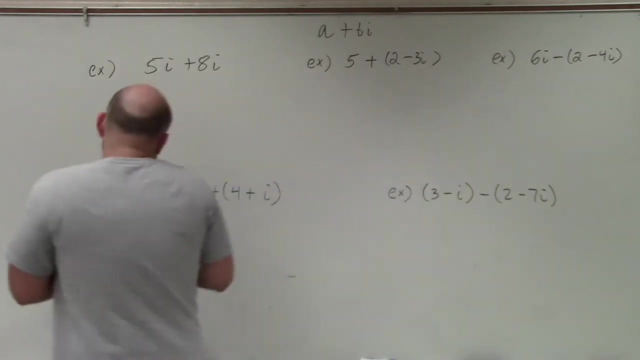 Or a number that had X's with the number, You could only add like terms. Well, when adding and subtracting complex numbers, it's the exact same. We can only combine real numbers with real numbers and imaginary numbers with imaginary numbers. So if we look at my first example here I have 5i plus 8i And what you can see in this case is these both represent. these are both imaginary numbers. So when we're adding them, I like to always think of this as it's like the same thing as saying: you know what is 5x plus 8x? 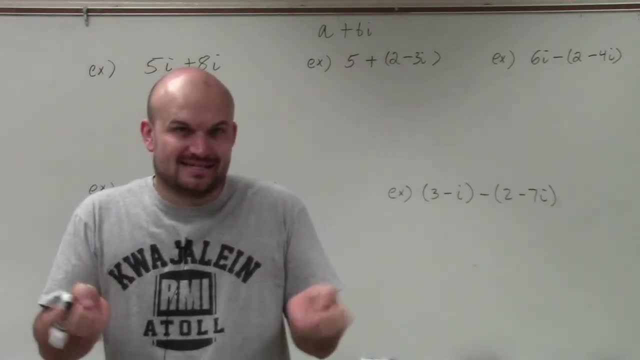 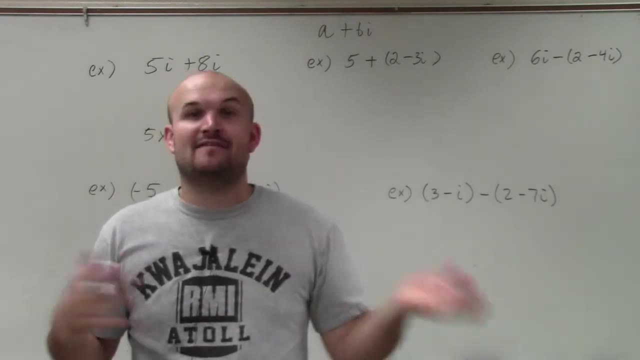 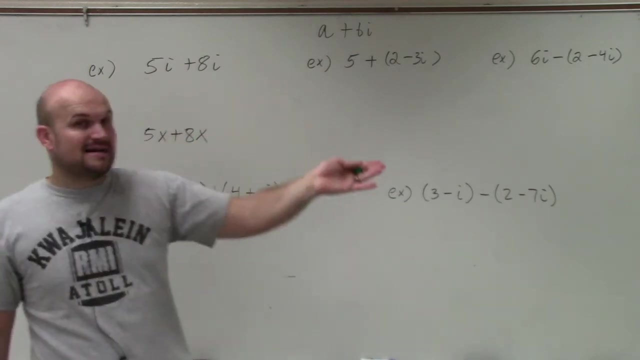 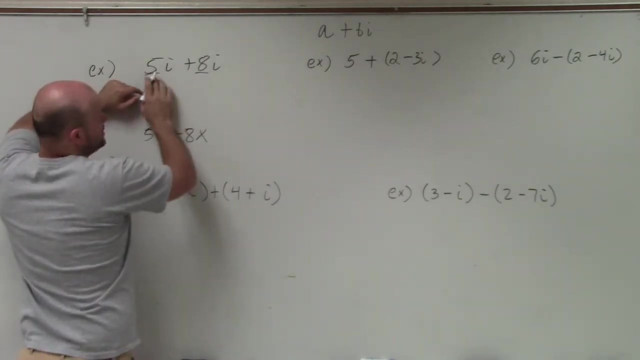 Or you know, 5 apples plus 8 apples, even though the X is an imaginary part, But it's the same thing. You're going to add the coefficients and keep the variable, OK. So that's why I give the example: 5 apples plus 8 apples. You say, oh, it's 13 apples, right? Well, X represents any number, I represents our imaginary unit. But still, when you're combining imaginary units, you just add your coefficients and you keep the imaginary unit. So 5i plus 8i is 13i. 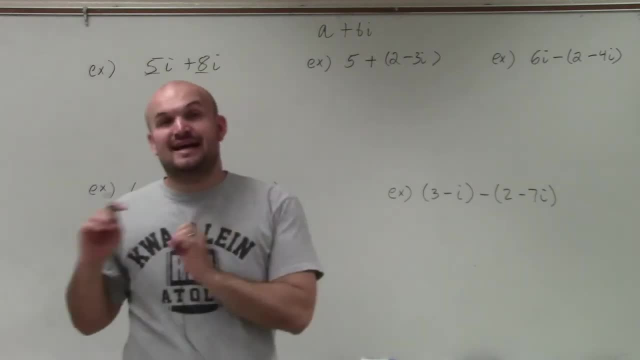 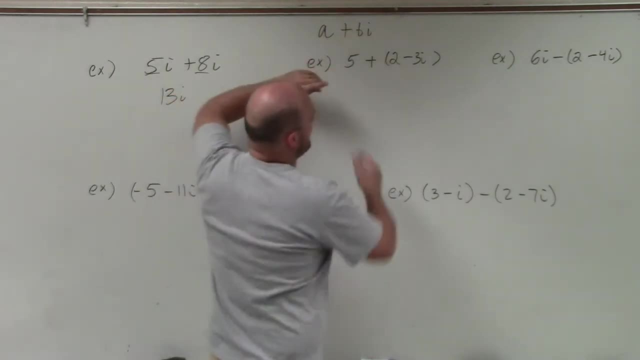 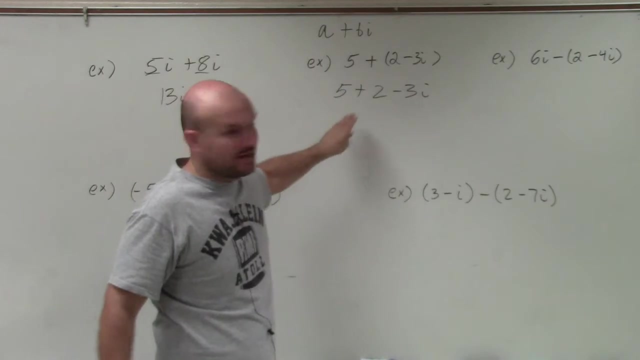 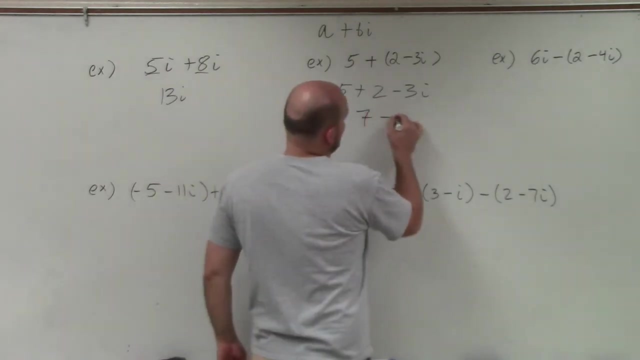 OK. So now we're going to start mixing our imaginary numbers and our real numbers, And in this case here I have parentheses, but I really don't need parentheses here, So I can just rewrite this without the parentheses: 5 plus 2 minus 3i. Well, you can see, I only have two real numbers, which is 5 and 2.. And I have my imaginary number, which is negative: 3i. So now I just add 5 and 2, which is going to give me 7 minus 3i. Done. 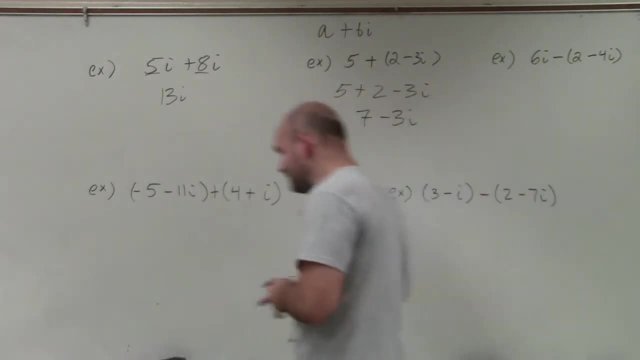 Over here. now. in this example, I have parentheses, but I'm going to need to apply this because not only am I subtracting the 2, but I'm subtracting the 2 minus the 4i. So what I'm actually going to do is I'm actually going to distribute this negative here. So therefore, I'll rewrite this as 6i minus 2i, and then minus a negative in terms to a positive 4i. So it's very important when you have a negative outside parentheses, that you make sure you distribute that. 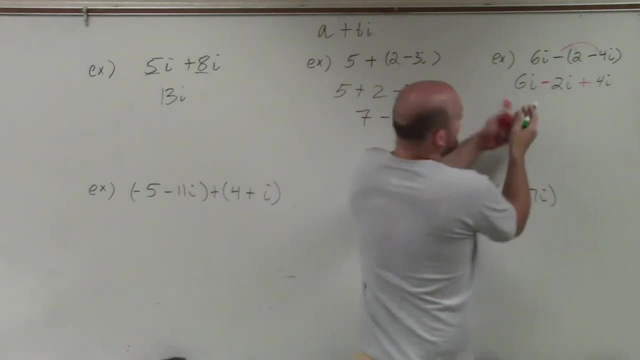 That's just the same thing, Yeah well, So therefore, now you can see, I have my imaginary units. Excuse me, Excuse me. So therefore, I have 6i minus 2i, which is going to give me 4i, and then plus. 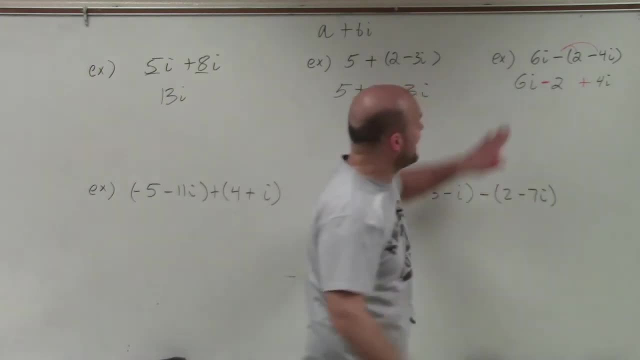 Oh, what am I doing? There's no i there, So therefore here I can't subtract 6i minus 2i. I just wrote an i there for some reason. So what I'm going to do is I'm just going to rearrange these. 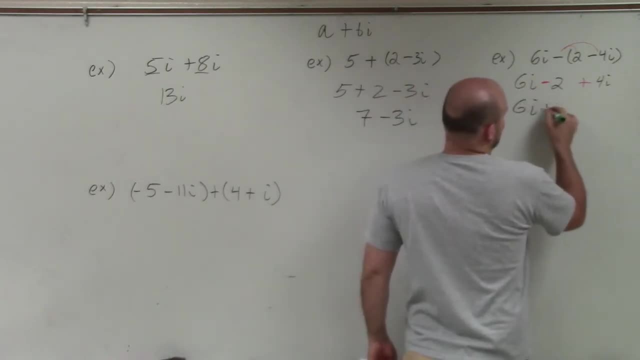 So therefore, if I use my periods, I get 6i plus 4i plus 1i. So therefore, if I use my terms, that's OK. So I'll rearrange this into 6i plus 4i minus 2.. 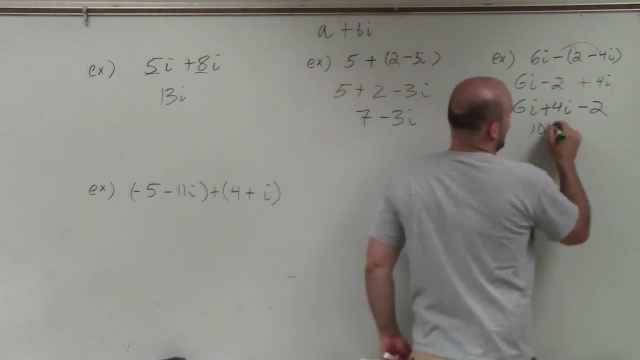 All right, So now I can combine these to give me 10i minus 2.. But remember, whenever we're writing imaginary numbers, we always want to write it in a plus bi format, So therefore I need to rewrite this as negative: 2 plus 10i. 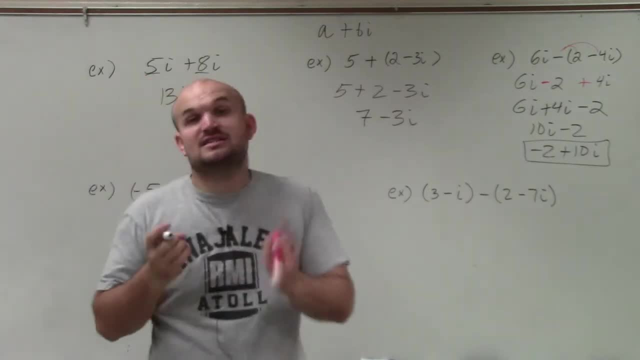 OK, We're always going to write it in that form where our real numbers is in front of our imaginary number. So even though, mathematically, if it was easy for me to re-write that about, I could write that down. 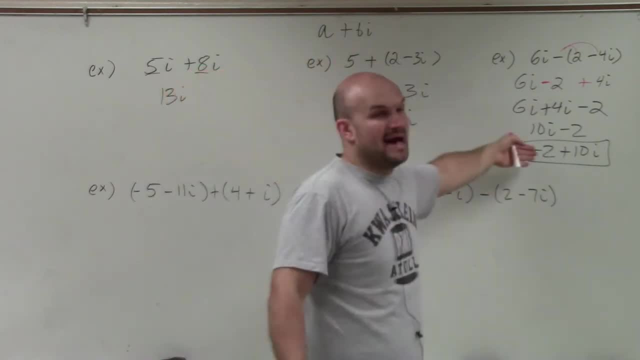 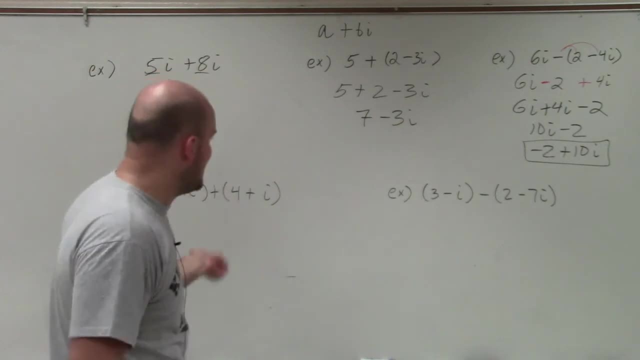 Alright, Sorry, That's aballs that way. I want to make sure I go back and rewrite it correctly. Okay, so now there's a couple different ways to do a problem like this. And now we have imaginary and we have real. 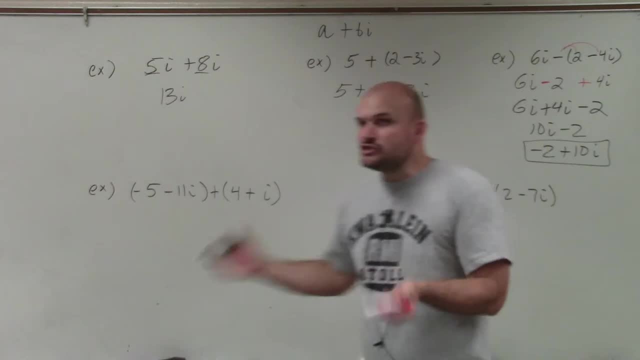 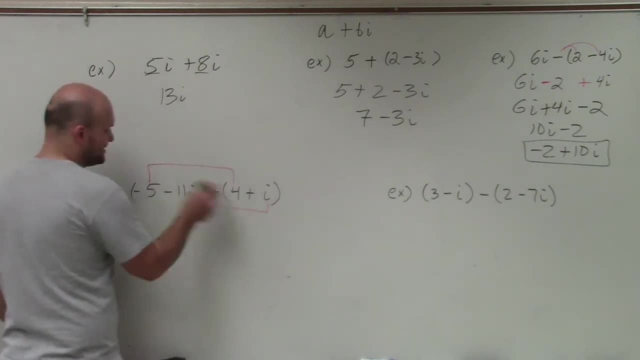 all right, And you can have. I'm doing an addition problem and I'm doing a subtraction problem. Usually with addition, I think it's just easier just to say: oh well, here's my two imaginary numbers and here's my two. here's my two real numbers and here's my two imaginary numbers. 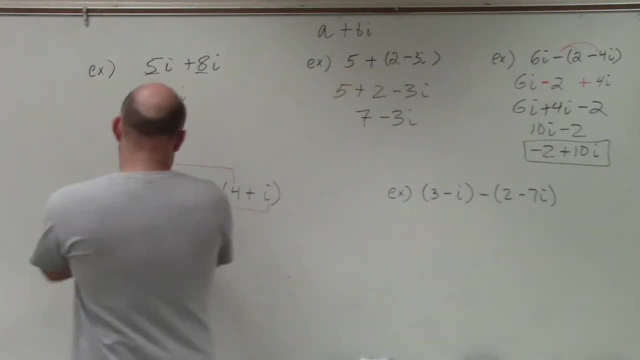 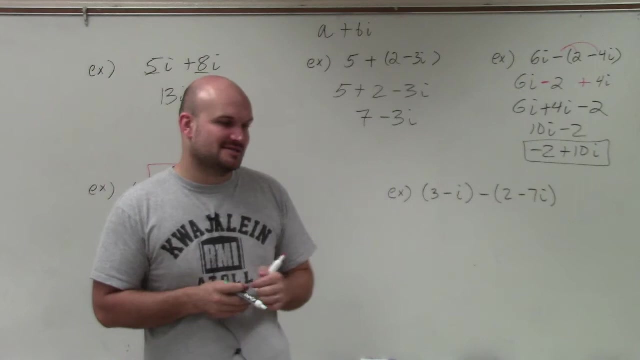 Take the signs that are in front and let's combine them, So I have negative five plus four. Well, that's going to be negative one. Negative 11 plus i is going to give me a negative 10i. Not really that easy, However, when we have subtraction again. what I like to do is 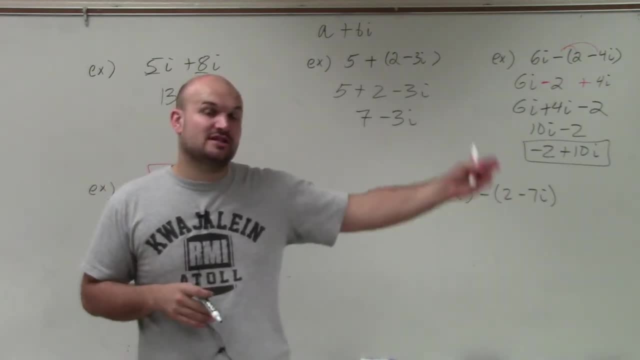 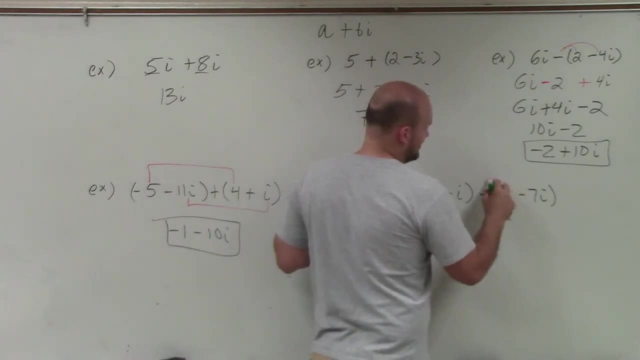 what I would say is: distribute this, make sure it's an addition problem, And once you rewrite it as an addition problem, then go ahead and do that. So again, we're going to distribute this, Okay. So therefore, it's three minus i minus. 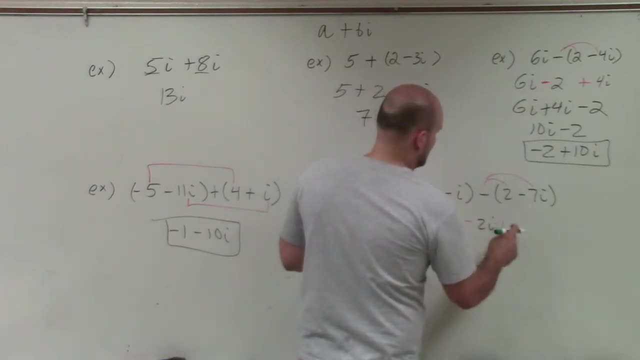 three minus i, Two i, and then plus seven i, And then I just go ahead and rearrange them again. Why am I doing this? i again. Why do I do that? It's just the negative you're distributing. So therefore this becomes three minus two minus i plus seven i. Well, three minus two is one.